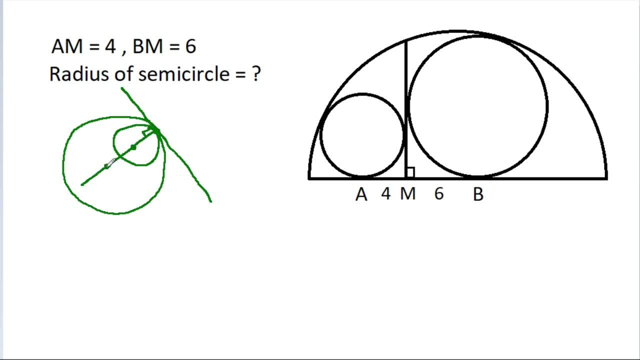 then it will pass through center of both the circles. suppose o and q And suppose the center of the semicircle it is o, This point is o, And suppose bo is x, then mo will be 6 minus x, because bm is 6.. 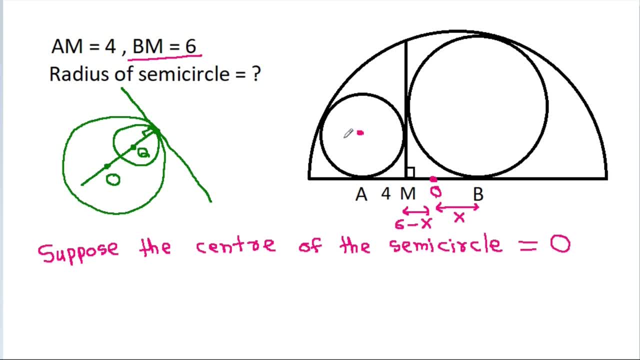 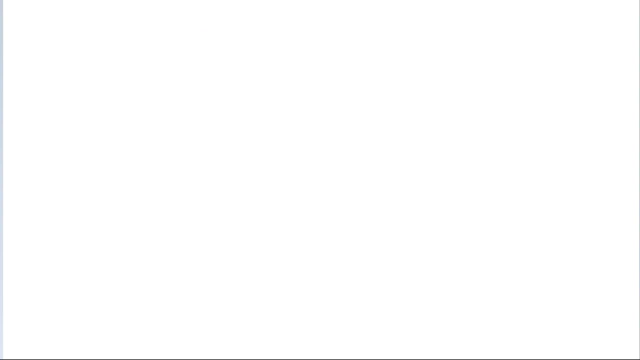 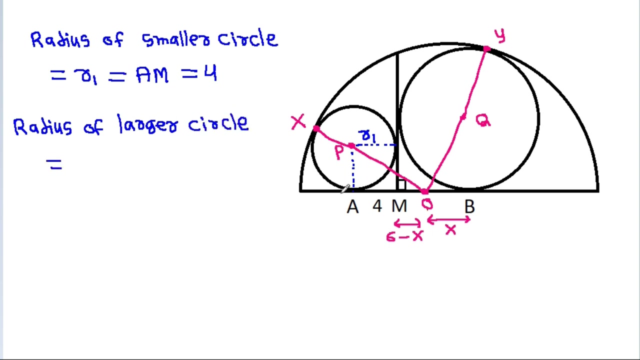 And if we join xp, then it will pass through o, And if we join xp then it will pass through o. Now radius of a smaller circle. Now radius of a smaller circle. Now radius of a smaller circle, Suppose suppose, Suppose it is R1, then it will be equal to AM, that is, 4 and radius of larger circle. 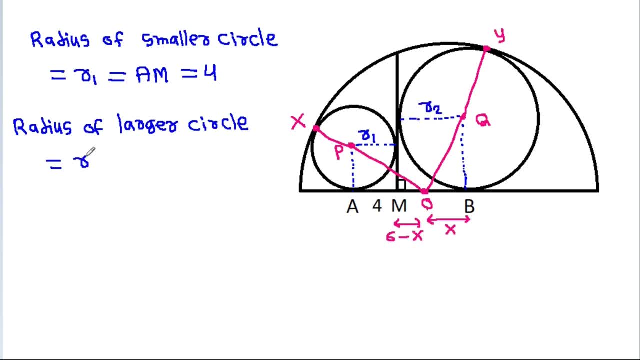 suppose it is R2, then it will be equal to BM, that is 6. and suppose radius of semicircle is R, then OY will be R and QY is R2. so OQ it will be equal to OY minus QY, that will be R minus. 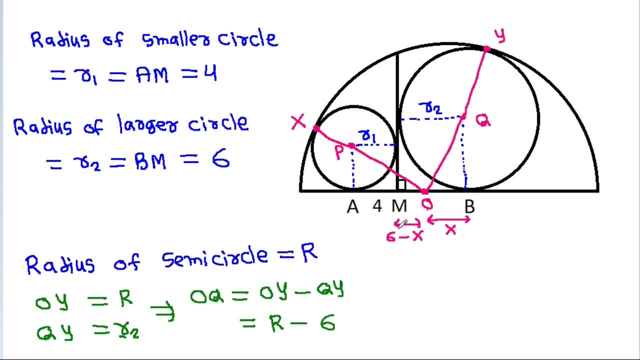 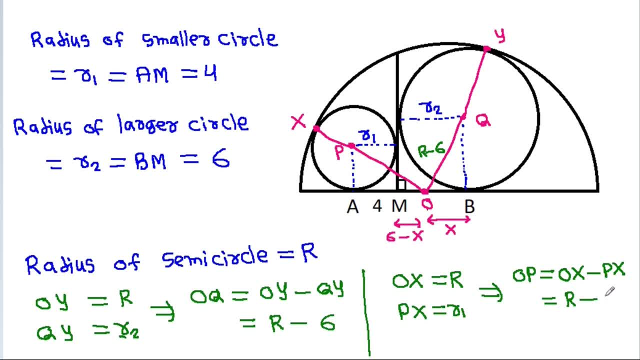 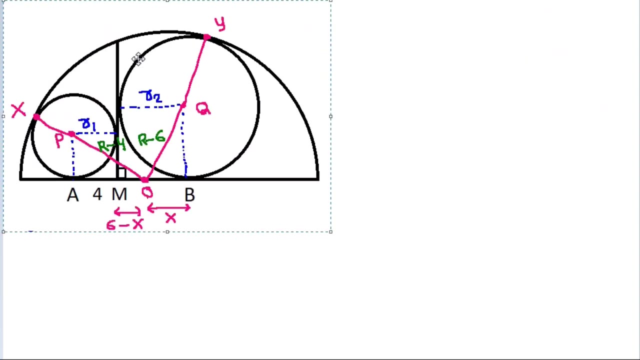 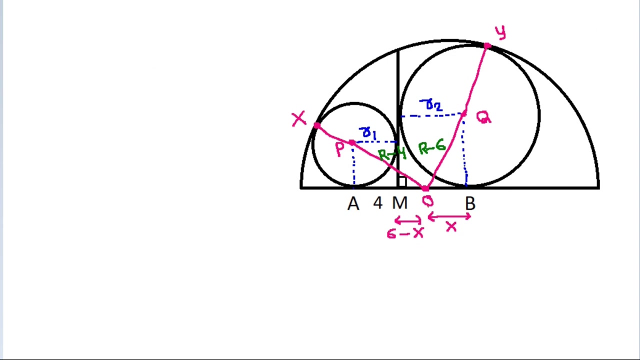 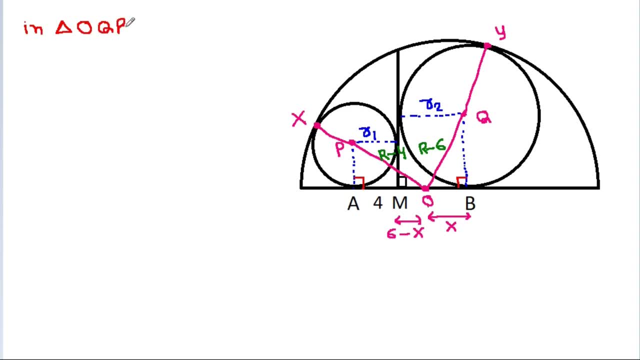 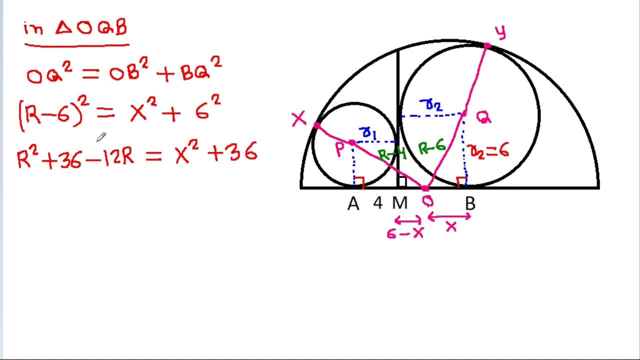 minus 36 and 36 will get cancelled. so x square is equal to r square minus 12 r and x will be equal to a square root of r square minus 12 r and in triangle, opa- opa squared, it will be equal to oa squared. 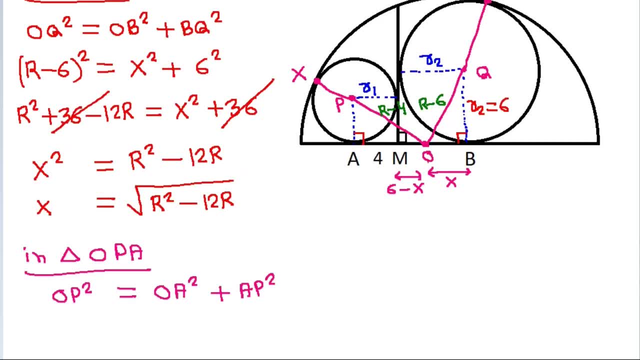 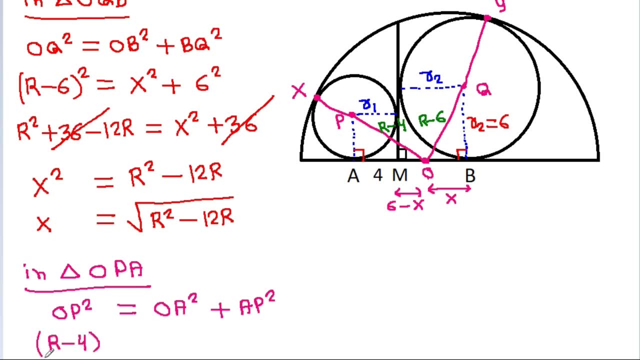 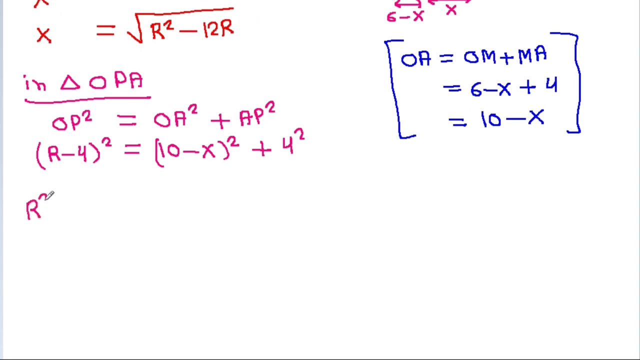 plus ap square and op is r minus 4 square. that is equal to oa. oa is equal, toikka is equal to om plus ma, and om is 6 minus x plus ma is 4 and it is 10 minus x. oa is 10 minus x square plus ap. it is r1. that is 4, ap is 4 square and it is r square. 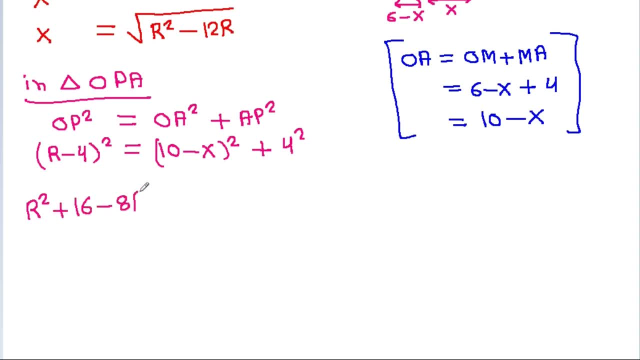 plus 16.. minus 8r is equal to 10. square is 100, plus x square minus, 2 times 10 times x will be 20x. plus 4 square is 16 and 16 will get cancelled. so r square minus 8r, it is equal to 100 plus and from here x square, it is r square minus. 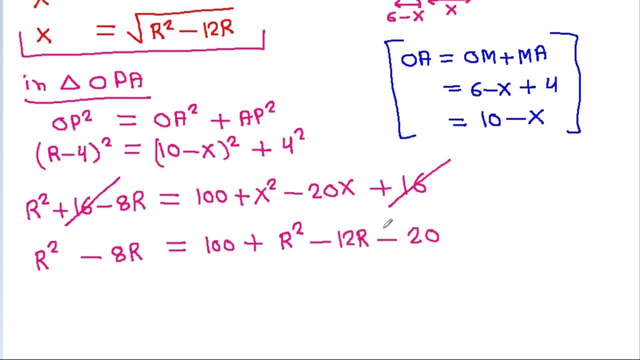 12r minus 20 times and x is square root of r square minus 12r and r square will get cancelled and minus 8r plus 12r will be 4r. that is equal to 100 minus 20 times x, square root of r square. 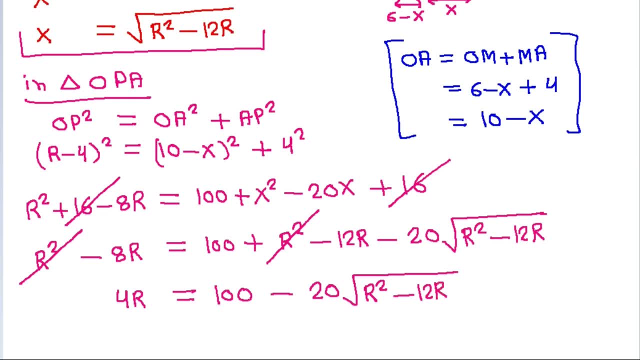 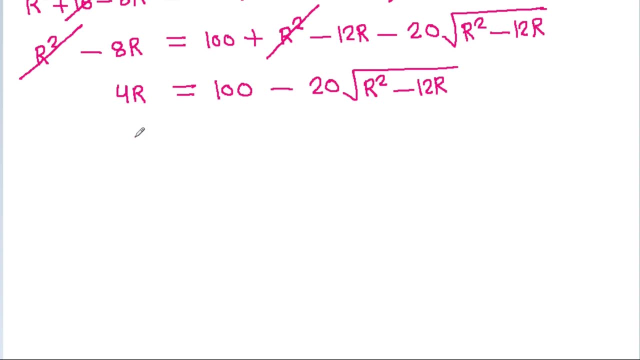 minus 12r, and if we divide by 4, then r will be equal to 25 minus 5 times x square root of r square minus 12r, and 5 times x square root of r square minus 12 R, it will be equal to 25 minus R, and if we square it both side, then this will: 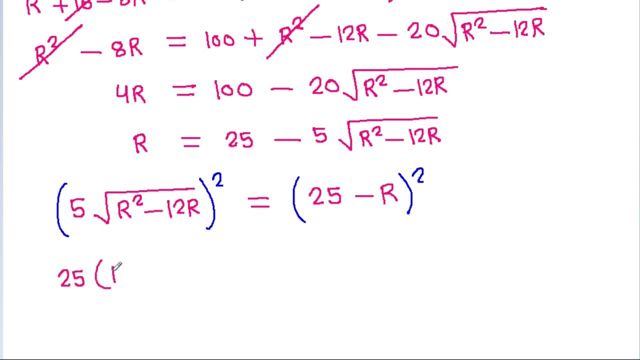 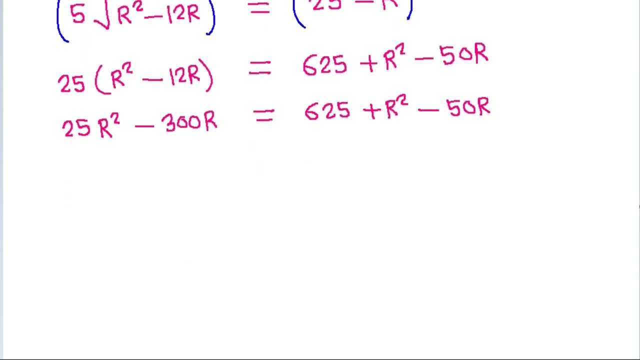 be 25 times R square minus 12 R, that is equal to 25. square is 625,. plus R square minus 2 times 25 times R will be 50 R, And it is 25 R. square minus 300. R is equal to 625 plus R square minus 50 R and 25 R square. 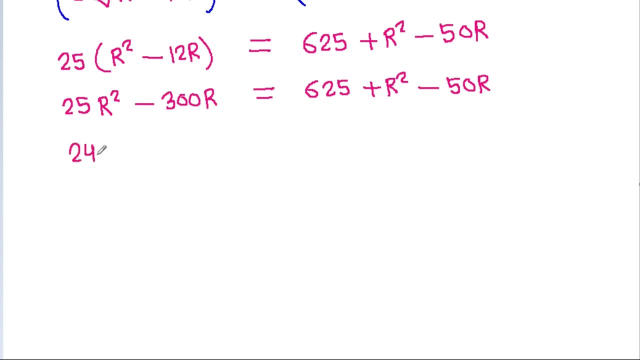 minus R square, minus 2 times R, R square will be 24 R square and minus 300 R plus 50 R will be minus 250 R. minus 625 is equal to 0.. And now we need to write: minus 250 R is AR plus BR, such that A plus B it should be equal to minus 250.. 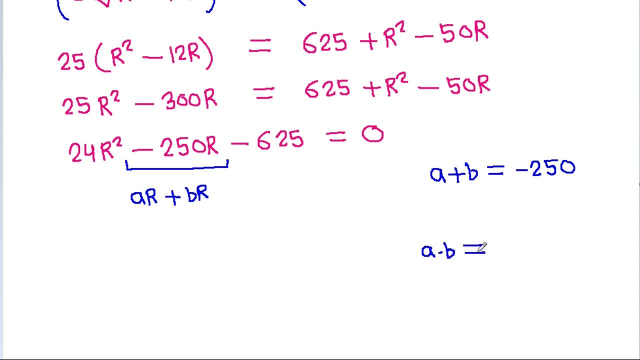 And A times B, it should be equal to 24 times minus 625.. 24 times minus 625- and it is minus 24- is 2 times 2 times 2 times 3, and 625 is 25 times 25, and 12 times 25 is 300, and 2 times 25 is 50. so it is minus 300 times 50 and minus 250. it can.